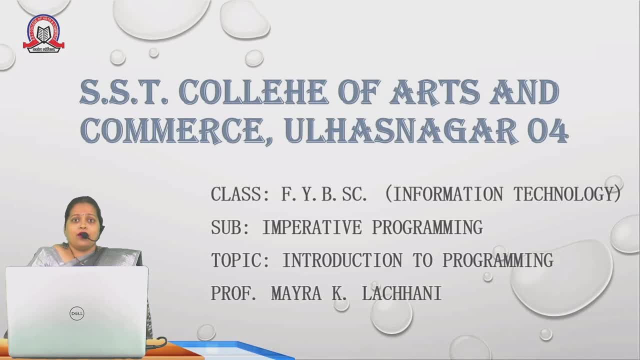 four digit pin or select your language or start your transaction. That means by reading those instructions. we perform accordingly. So these kinds of applications are called as console application. Next is windows application. Windows application means where you will get executable file or setup file which we can install in particular window or in any other. 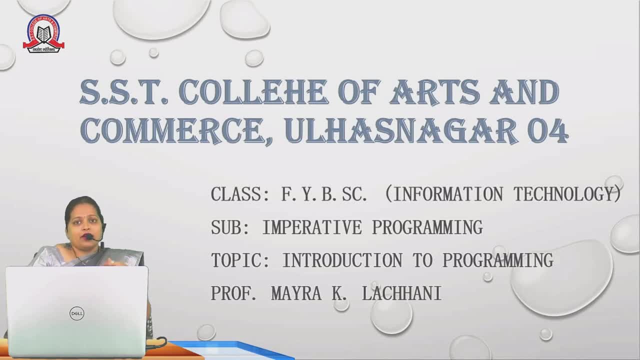 application. You can install these applications in your application and you can also use it, or in machine where that application will run like, suppose we can say, a microsoft office. or here in c programming we have to use turbo c application. these applications are called as windows application. next is web application. web application means which runs on internet or on 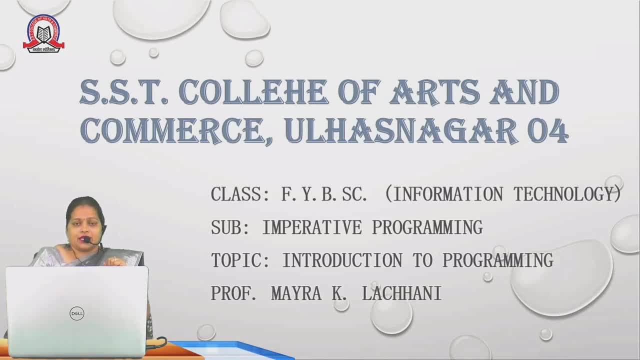 browser. to execute or to run any web application, we we need two things: one is browser and another is internet connection and last one is mobile application, which we use in our daily life. so let's start with a session that is c programming language. here, first of all, we have to learn about 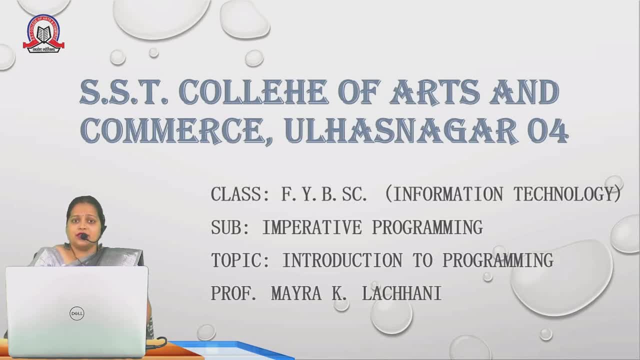 abcd, abcd of programming. abcd of programming means, if suppose we'll take example of english language, even in that language we have to learn about abcd. then only we can write or we can read apple. so we have to learn about abcd, then only we can write or we can read apple, so we have to learn. 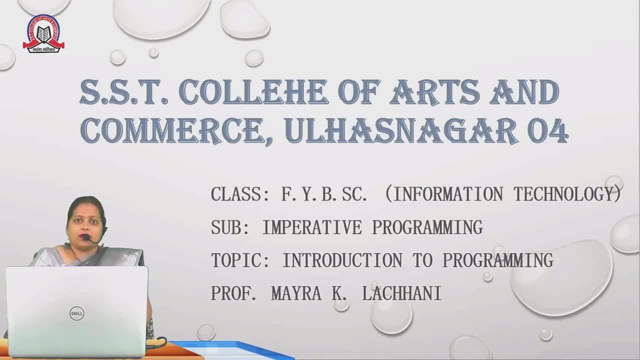 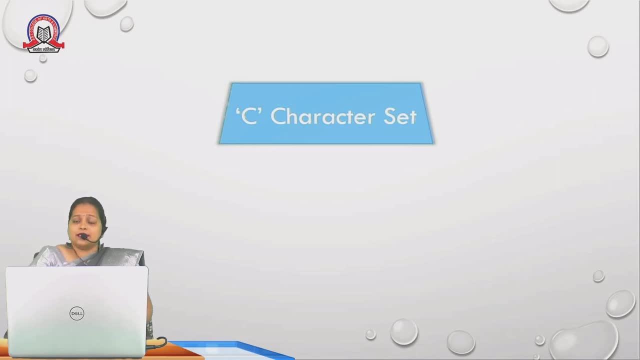 about abcd. same like in programming language. we have to learn about abcd of programming. so first of all we'll see character set c. character set means using these characters we have to write our program. so what are they? we can use capital a to z, small a to z, 0 to 9 and combination of: 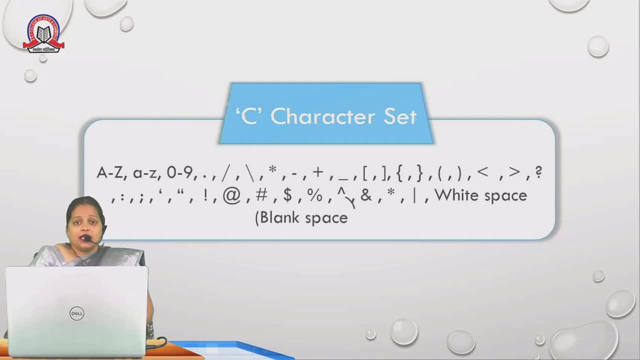 all these alphabets, as well as digit. with this we can use all the special symbols which are present on our keyboard, including blank space, which is also called as white space in programming language. so these are character set which we can use in our program. next is token: whenever we'll. 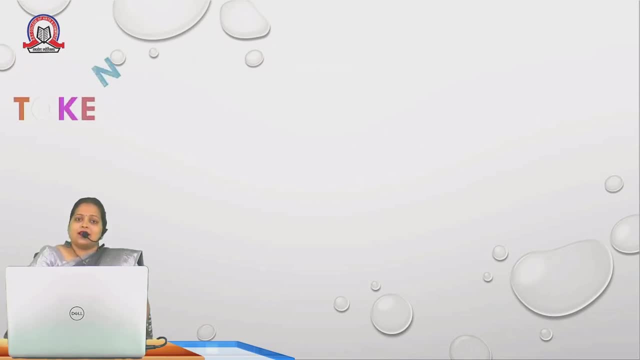 write our program, we'll use tokens. there are five different types of tokens, but before that what is been the token? the smallest individual unit in a program is known as token means. if suppose we are writing a program or we are writing a code which is of hundred lines or of hundred words, so from those words we call an individual. 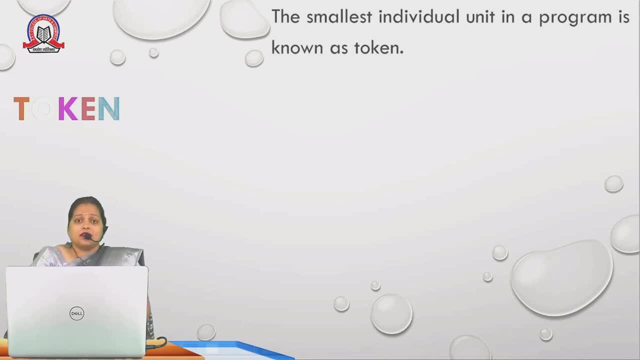 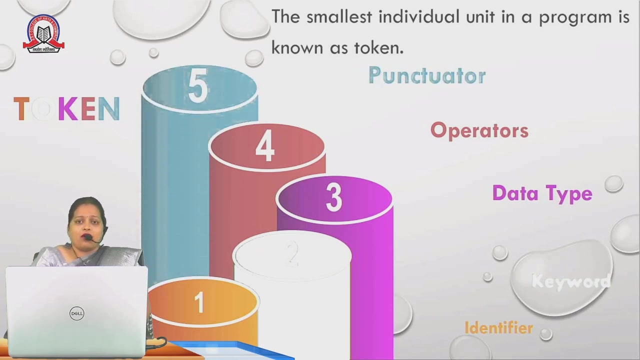 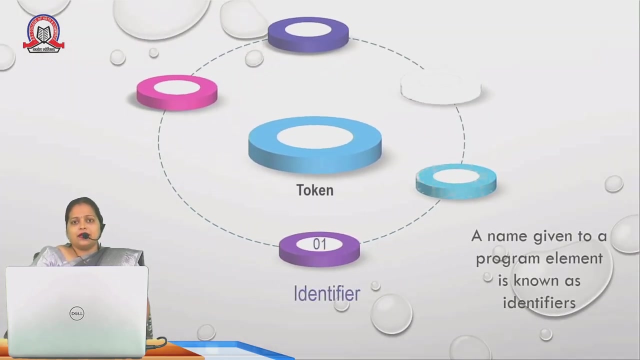 word as token. so what are the five different types? one is identifier, second is keyword, third is data type, fourth is operators and fifth is punctuator. so we'll see this: all identifiers one by one. first is identifier. identifier means a name given by a person that is given to a program element. now, if we want to understand this in detail, then 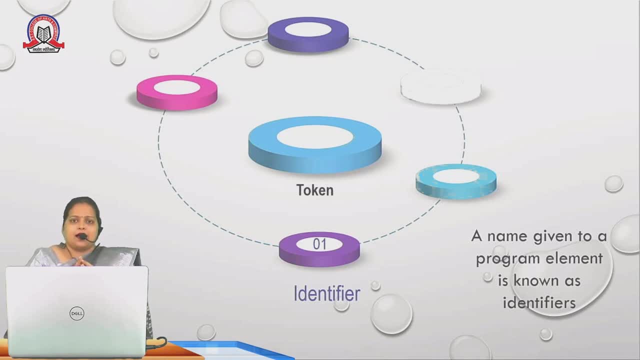 we'll take one example. if there's a new born baby in our house, then we give it a name. we give that name so that we can identify that child, we can call that child. so to call that child, we give it a specific, unique name. similarly, in programming language we have to give a unique. 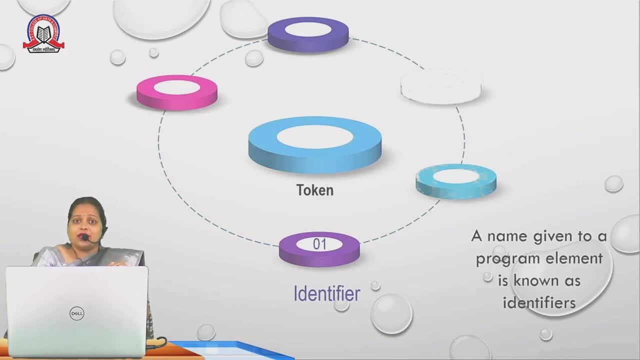 name which we value on this particular memory, so that we can identify that child, we can name that child in our program, and in our program we name that child in our program store karni hai. uss memory ko naam dene ke liye, we use identifier. next is keyword keywords. 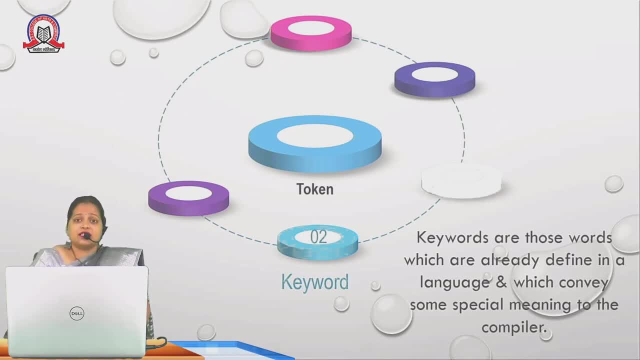 are those words which is already defined in a language and which convey or which carry some special meaning to the compiler. now, who is compiler? who compiles or who execute? our program is known as compiler. so like abhi hum log ne previous identifiers me example liya tha new born baby ka. to new born baby ko hum log ek unique naam dete usko hum log. 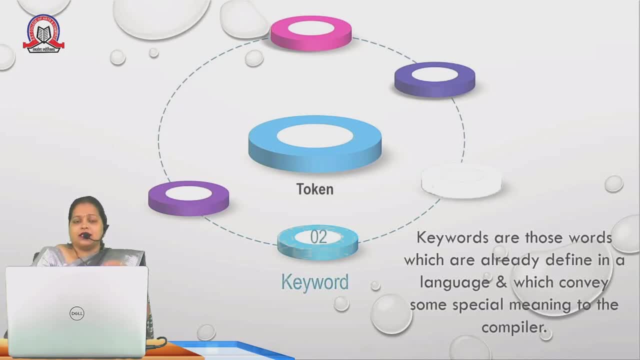 girl ya boy ye name nahi dete kyu, because in our dictionary ya humare language me girl or boy, ye word ka ek specific meaning hai. to vo meaning hum log ko kuch batata hai. to vo meaning jo hai vo hum log kisi bache ko naam, ya unique name dene ke liye use nahi. 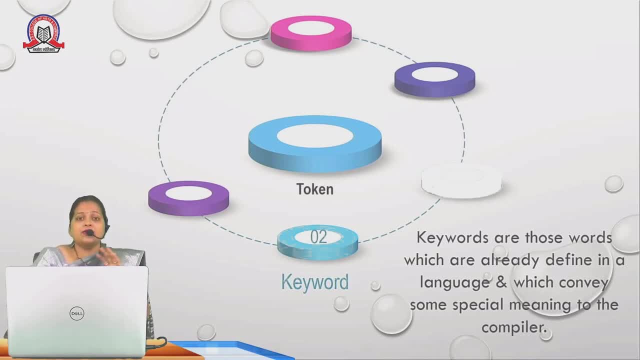 kar sakte. waise hi, in programming language we cannot use keywords as an identifier, because compiler ke pass keyword ka ek already ek meaning hota hai, so hum log usko ek memory ko naam dene ke liye. we cannot use keywords as an identifier, waise hi identifier, declare karne ke liye, or identify, define karne ke liye. there are five. 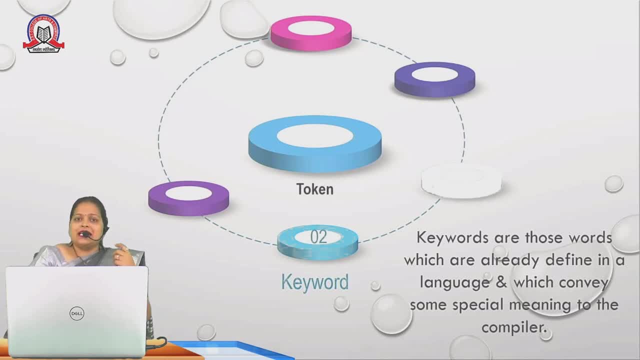 rules. there are four rules. which are them? it contain capital a to z, small o to z and zero to nine, but it should start with alphabet. we cannot give blank space in between identifier, so instead of a blank space, we can use underscore. and the very important rule is we cannot give. 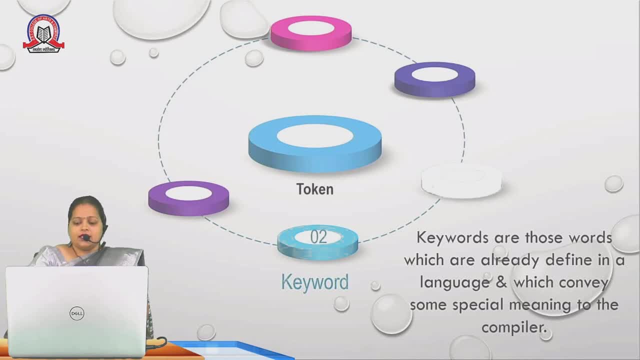 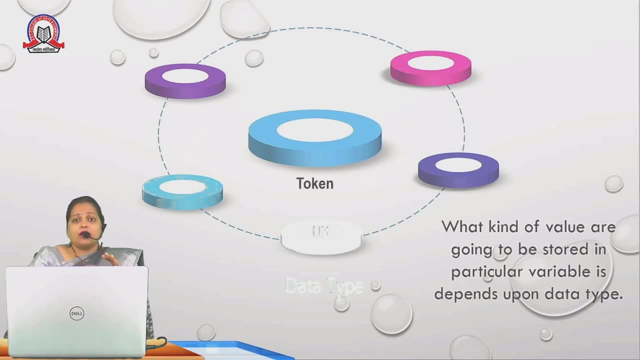 blank space in between, and we cannot use keyword as an identifier. the next token is data type like hum log ne memory allocate kar liye. now what kind of value are going to be stored in that particular variable is totally depend upon your data type. there are three types. 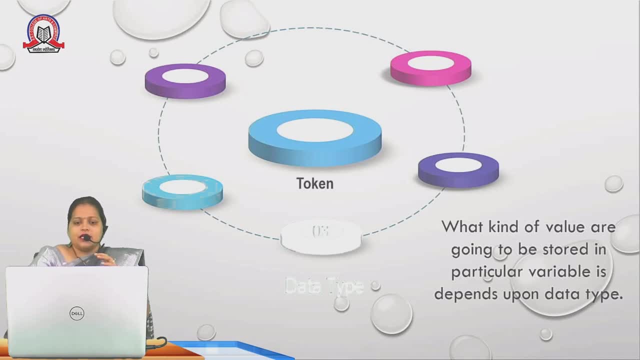 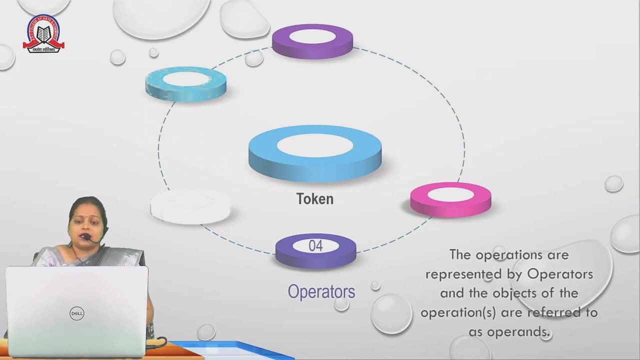 of data type that we will see in further slide. next is operators. the operations are represented by operators and the objects of the operations are referred to as operand. even there are three types of operands that we will see in further slides, but operand ka hote, which is work on. 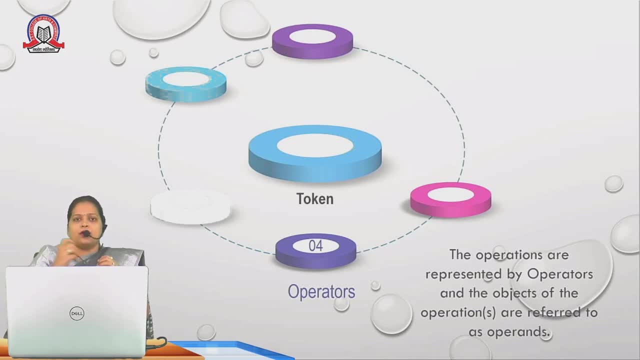 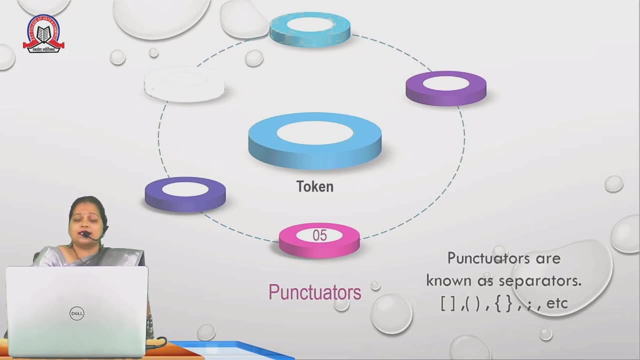 some values or some variables usi ko programming language me operands bolte hai. next, last but not the least, is punctuator, which is also known as separator. like two words ko hum log ko separate karna hai, we give comma. two sentences ko hum log ko separate karna hai, then we can. 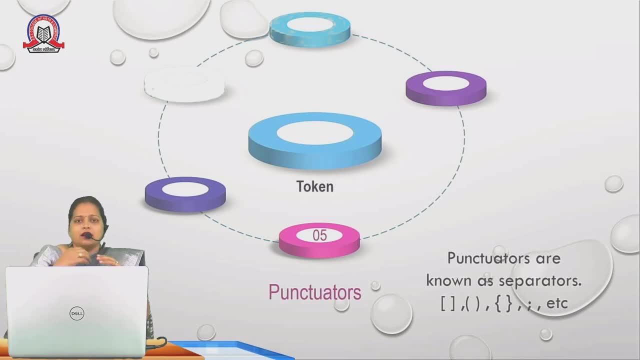 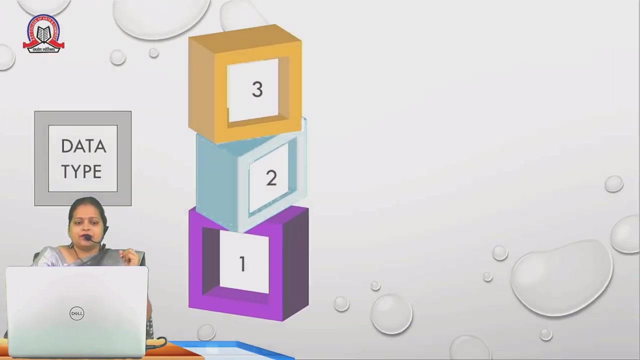 use semi colon. yes, in programming language to separate two sentences we have to use comma semicolon. Then we can separate two blocks with the help of curly braces. So these separators are called as punctuators. So we will see next data type in detail. There are three. 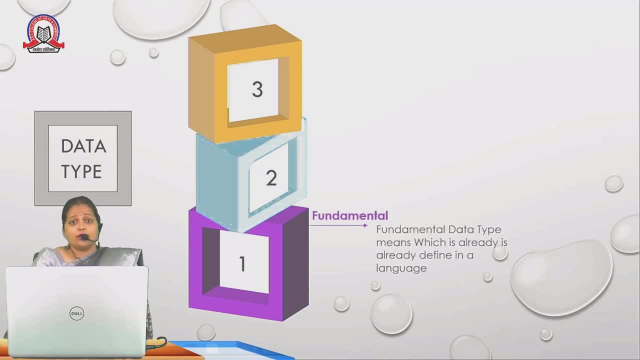 types of data type. One is fundamental, which is also called as predefined. Now, predefined means which is already defined in a language. Like we have seen the keyword which is already defined Compiler knows its meaning. Similarly, fundamental or predefined data type means which is already defined in a language. We can directly use it in our program, Like, suppose. 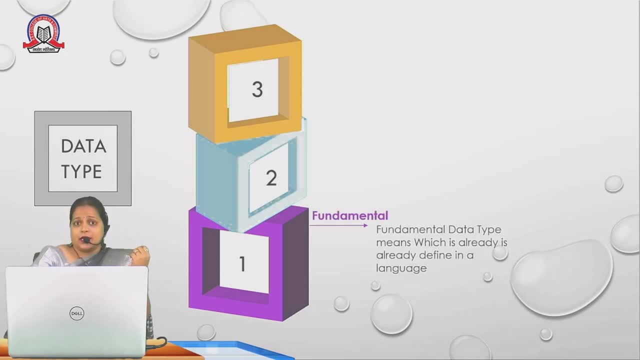 if I want to store a whole number, I can use integer data type. If I want to store a character, I can use char variable. If I want to store a decimal value, I can use float data type. So this is all about fundamental or predefined data type. Next is user defined data type. 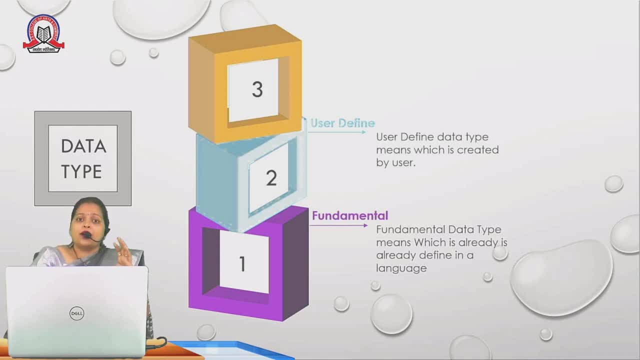 Now, user defined data type means user or programmer. Programmer will decide what kind of value are going to be stored in that particular variable. It depends upon programmer. It's called as user defined data type Example classes union that we can see in further in our subject. Next is derived: Derived data. 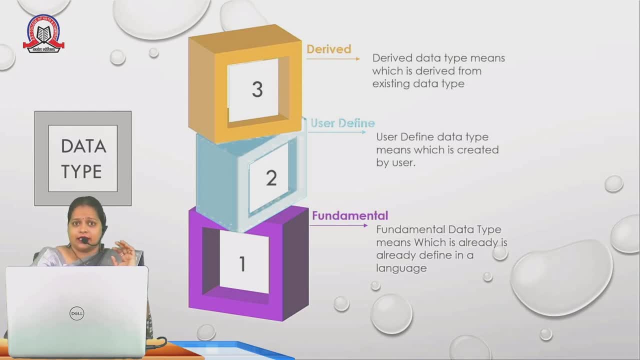 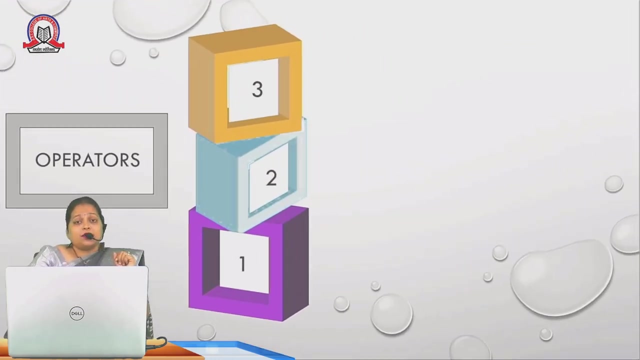 type means which is derived from any existing data type. It can be a fundamental or it can be user defined data type. Example: array and function are the same, They are all the same. So, again, this topic will explain in our further lectures. Next is operators. There are three types of operators. First is unary operator. Unary operator. 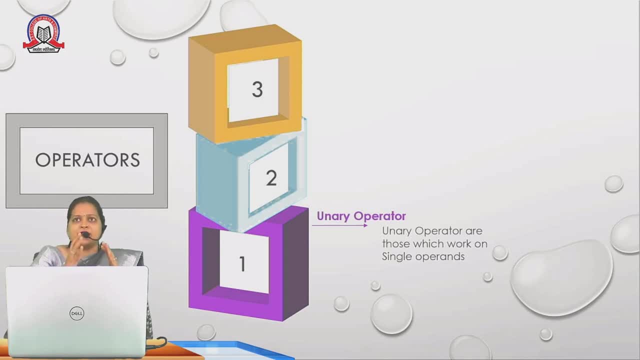 means which works on single operand. Single operand means if I want to show, or if I want to show a positive value or negative value, that we can or we can represent that with the help of like: if the I want to show 10 value that is positive, So I can write plus. 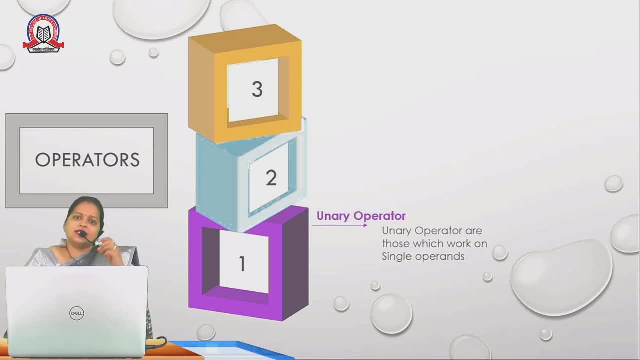 10. So this plus operator is working on single operand, that is 10.. Single value, that is 10.. So this operator called as unary operator means those operator which works on single operand are called as unary operator. Next is binary operator which works on two operands. 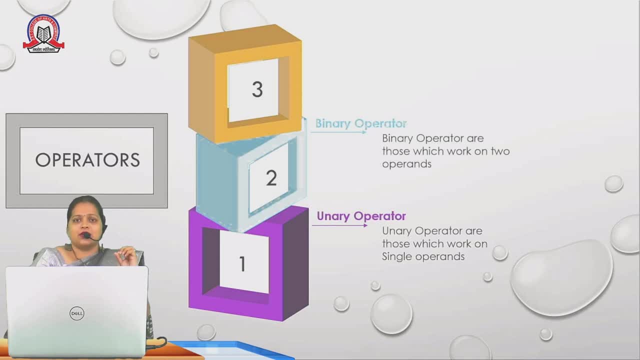 Like suppose we are writing expression like: c is equal to a plus b, So this plus operator is working on a and b. or else we can write: c is equal to 10 plus 20.. So this plus operator is working on 10 and 20.. So this plus operator is working on two values. That is why it is. 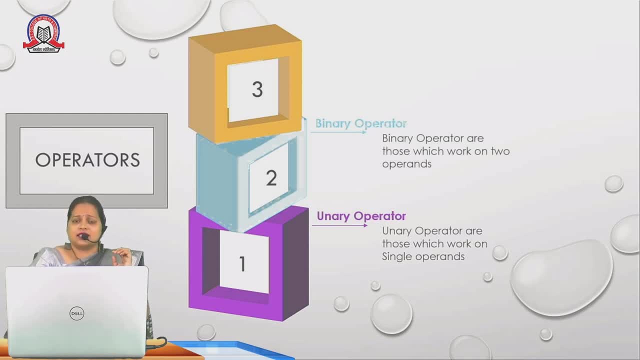 called as binary operator. Again, there is a further classification in binary operators. There are assignment operator, relational operator, logical operator. that we will see with the help of examples. Third is ternary operator. Ternary operator means which works on three operands. The operator is question mark and colon, which is also called as conditional. 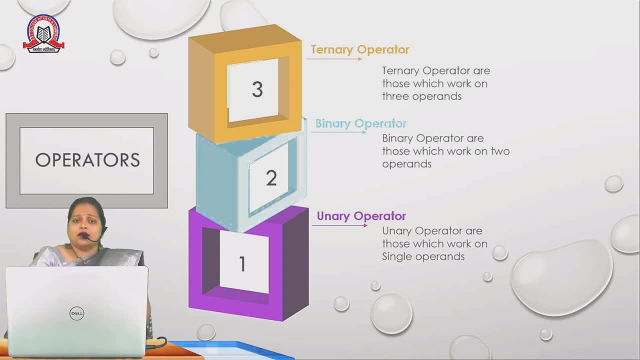 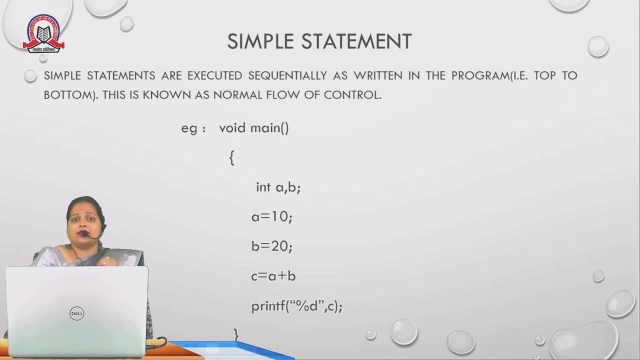 operator. Now we can see one example that is simple program. Before starting this explanation, I want to tell you one thing. There are four types of statements. One is simple statement, which is also called as sequence statement. Second is selection statement, where we can. 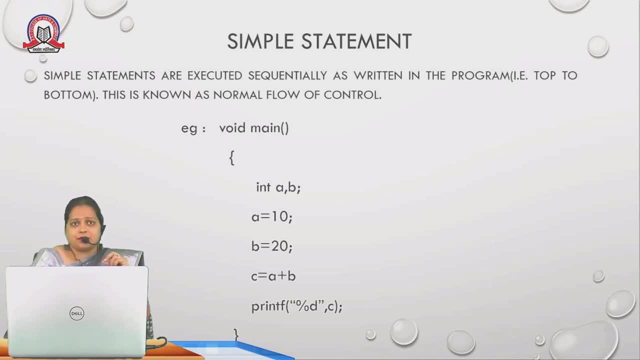 do conditional statement programs. Third is iteration statement, where we will do looping programs, and fourth is germ statement. So today we will see about simple statement or sequence statement. Simple statement or sequence statement means one by one statement compiler will execute. So here is one example In C programming language. whenever we execute, 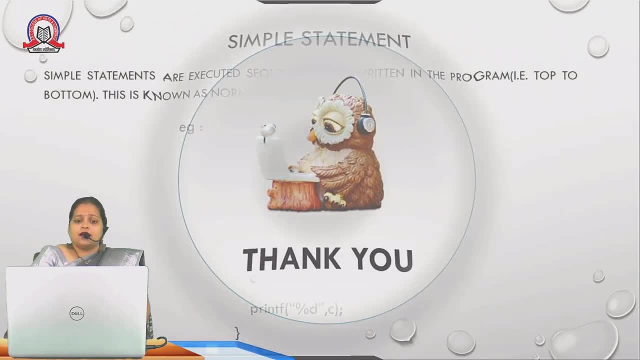 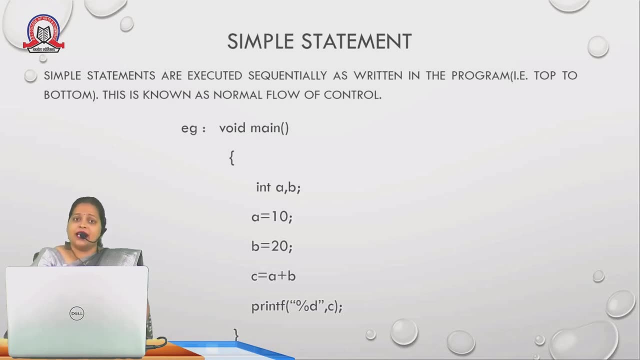 the program compiler, first look for the main function. Where is the main function? Because execution begins with main function and it ends with main function. So here is my main function. In that main function I have declared two variables. First one is function, Second one: 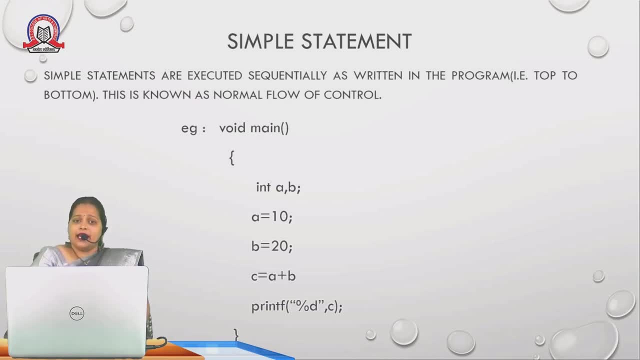 is function. Third one is function. Fourth one is function. Fourth one is function. Fourth one is function. So here I have declared a variable of integer type a and b. That means, in this variable I am going to store a integer value. That means whole numbers, Like here I have declared: 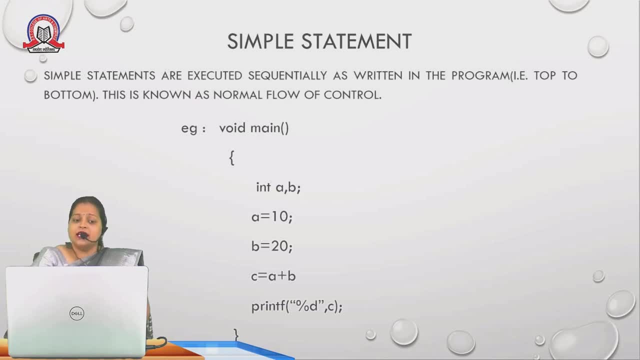 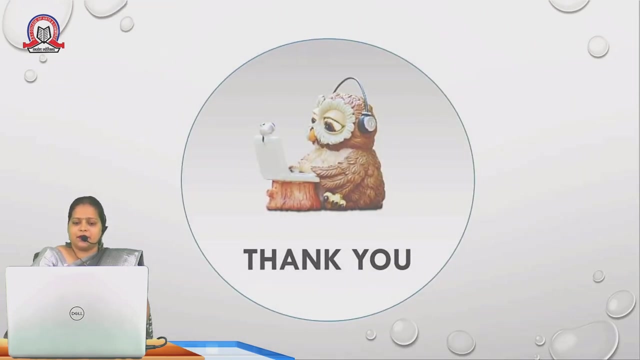 one or two variables, a and b, and here I am initializing this 10 value in this a variable and 20 value in this b variable. And here I am adding this two variable and storing that addition into the third variable, that is c variable. And here I am displaying the 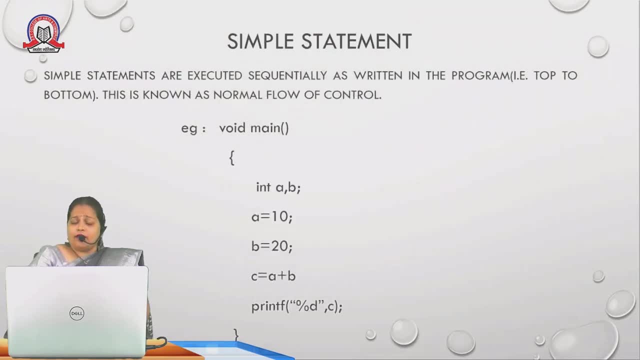 answer That is value of c Same. this thing we will do or we will see with the help of our program. So this is my program. These two statements are called as header files. This hash symbol represent this is preprocessor directory and include means we have to include. 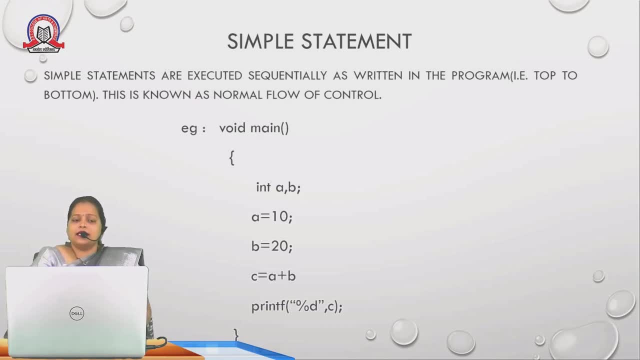 these two header files in our program. Okay. stdioh stands for standard input output operations and coniu stands for console input output. This is my main function. Whenever we will execute this program, compiler will start with main function. Here I have declared two, three. 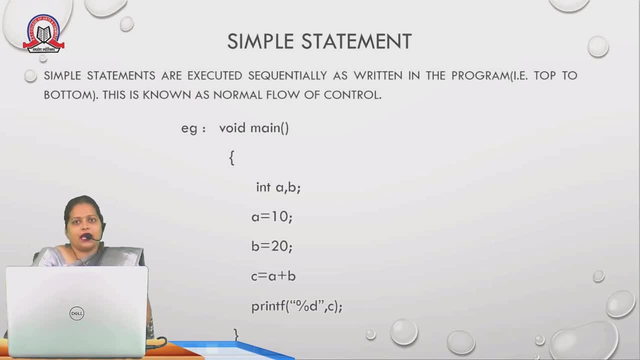 variables of integer type a, b and c. This is clear screen. This is clear screen. What does clear screen function do? It will clear our previous output on the screen. We will see that, along with executing it Here, I have initialized a variable. 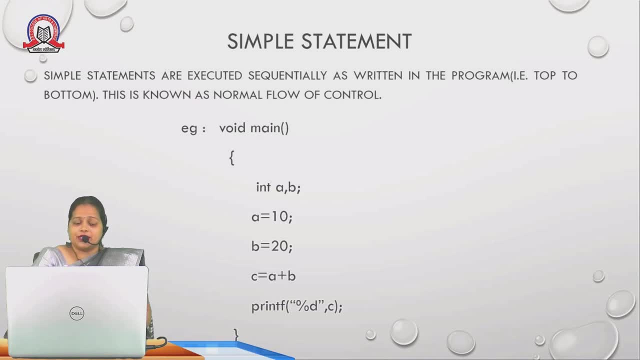 as 10 value and b variable as 20 value. And here, in c variable, addition of a and b variable is stored, which I am displaying with the help of printf function. So addition is equal to whichever is written inside the variable. So this is the printf function, This is the 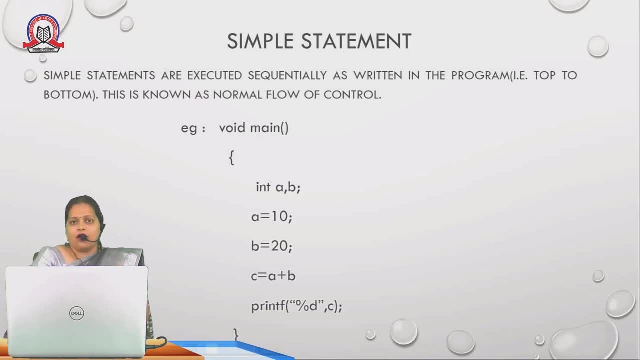 return inside the double quotes, It will print as it is on your output screen. So addition is equal to as it is print on output window and along with that, value of c variable will also be printed. I will execute this program for you. So here we will start execution of. 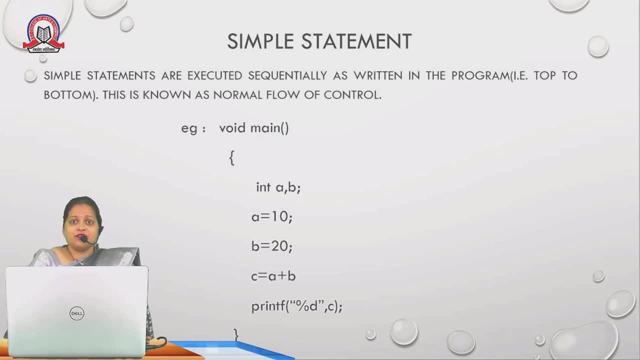 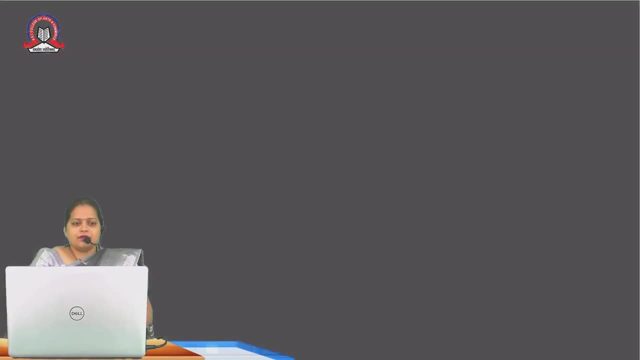 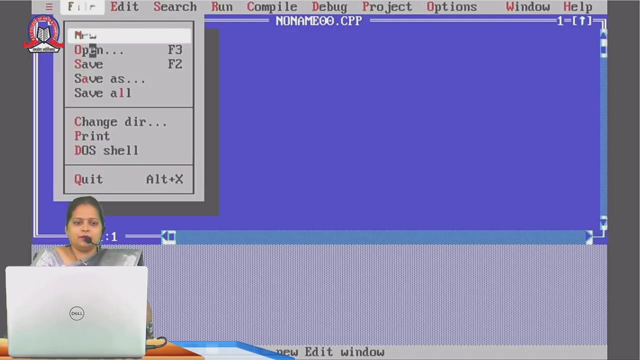 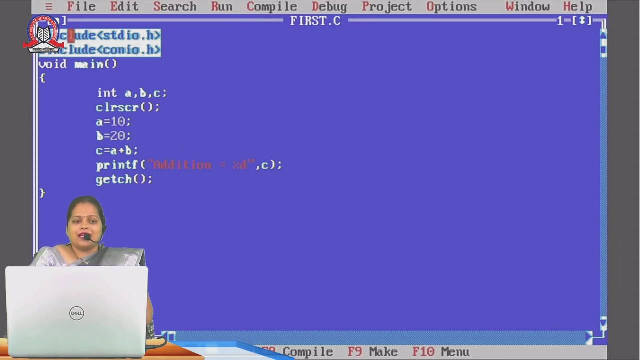 our program. So to execute c programming language we have to use turbo c application. So you have to click on start turbo c. I have written the program beforehand, Otherwise we can, or we can write our new program. This is my program, The first two statements, which is called header file, Here the hash symbol. 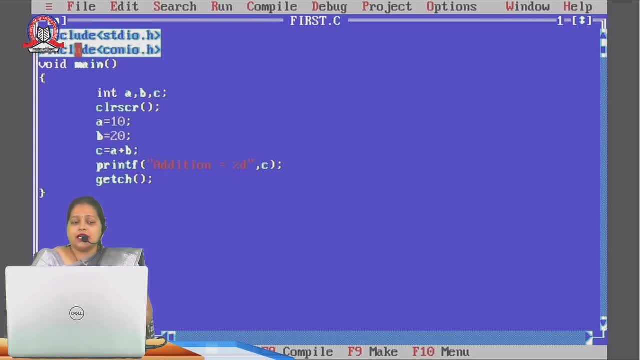 is visible. This is for: like: this is a pre processor directory For this. here a hash symbol is written. I have to include these header files in my program Because there There are some predefined functions for which I have to take permissions from the compilers. 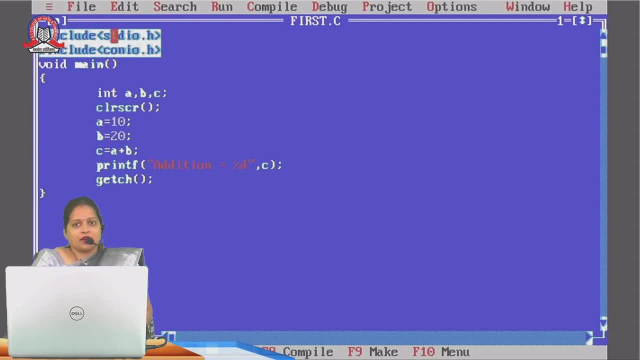 To execute those programs I have to include respective header file in my program. So stdioh stands for standard input output and conio stands for console input output. Console means our output screen. So here is my main screen main function. as like earlier I have said, told you that in. 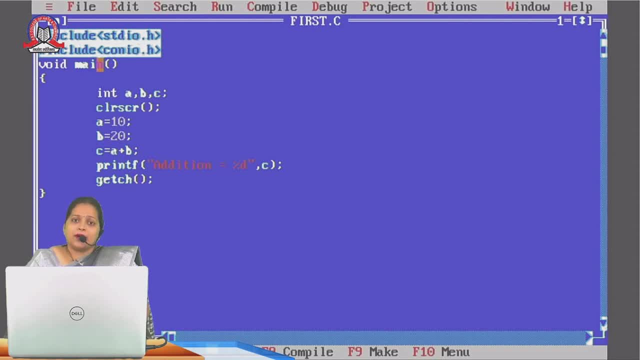 C programming language. whenever we execute our program compiler, first look for the main function. So here is my main function. execution starts with main function and it ends with main function. Here I have declared three variables of integer type. like I can store a whole integer numbers, 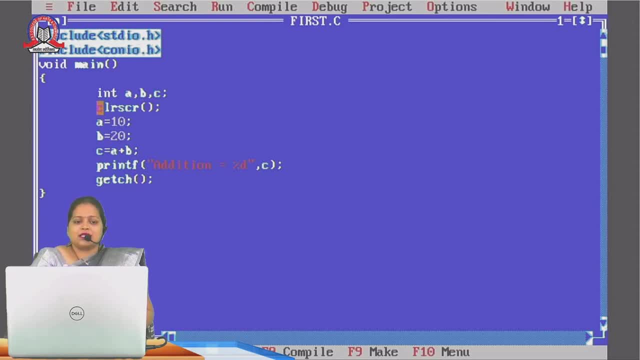 or whole numbers in this variables a, b, c. after this clear screen is written. This function comes under conioh header file, which we use because in previous output screen I don't need any message in this program output. if I want new output screen, then we. 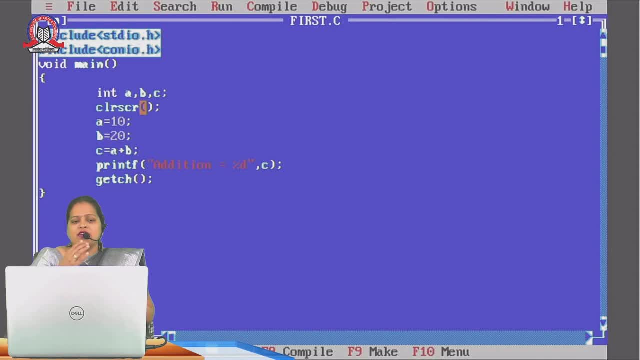 use this clear screen function over here to clear. Then after that I have initialized this 10 value in this a variable and in b variable I have initialized 20 value and then in c variable I am storing addition of a and b variables And after that here I am displaying or I am showing the answer, that is, addition of two. 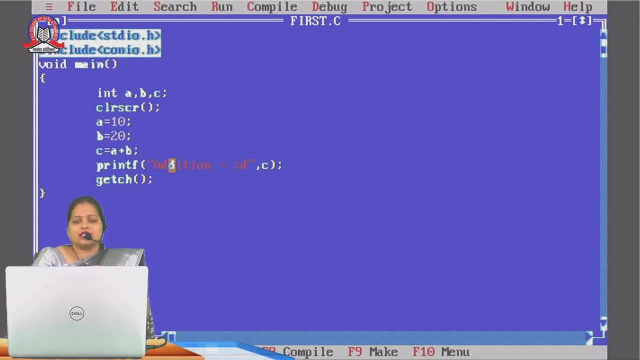 variables. So whatever is written inside the program in this variable will be an integer inside the double quotes it will print as it is on your console screen. that means i have written addition is equal to. so as it is up your output screen will print: and then value of that c variable. 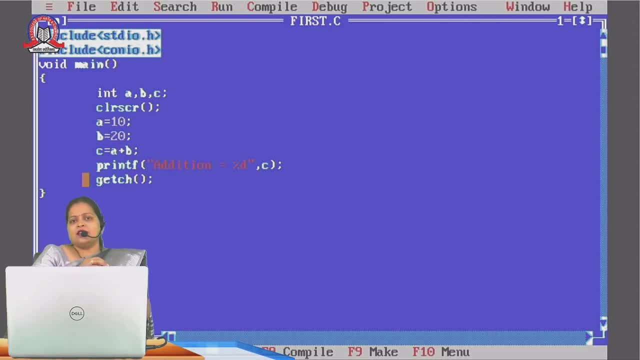 then get ch function. this function is basically for accepting a single character. but why we have written this function over here? because we will not call this function here. so output screen will hold the car by, because turbo CA application as a hey, jump up the program and up the output. a key. 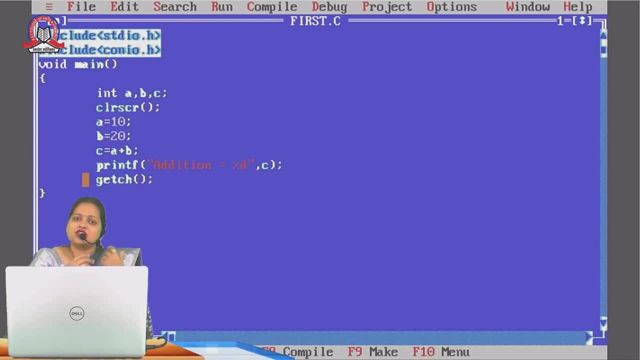 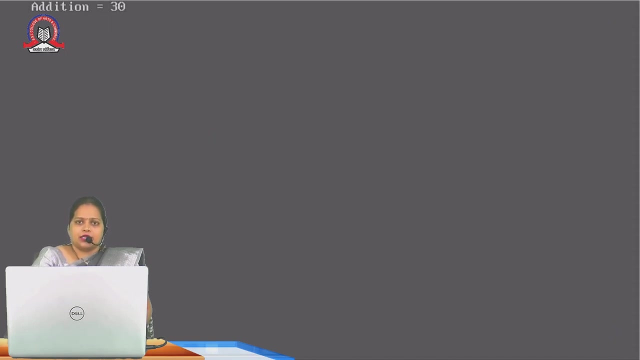 window pay at the top casual output window. a walk, a fraction of seconds, which Allah Jai go to to hold that output screen. we are calling this. get says function at the end of our program. so I'll execute this program. here is the answer. addition is equal to 30, up just a minute below the clear screen, a. 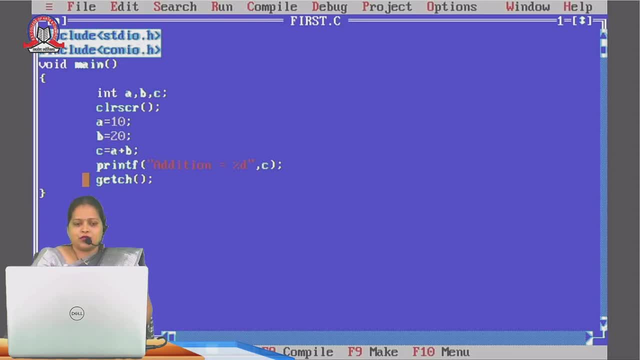 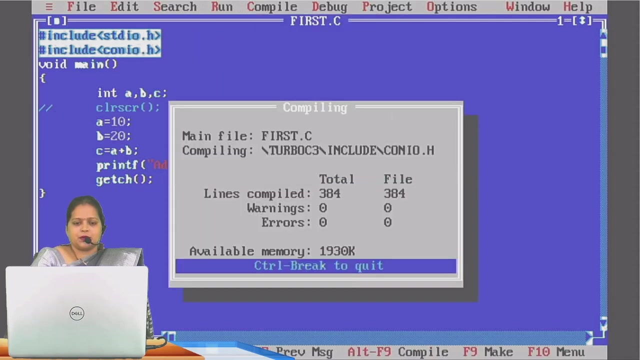 joke. function here is complegna is really good. you can previous output religion each I hear. so is function on the hopper comment: cut the comment in the sense is Istia. function of board. Mayamla quote the grain, but compiler was cultural aBL. that means yes, function. joy will execute the yoga. now let's execute this program. see. 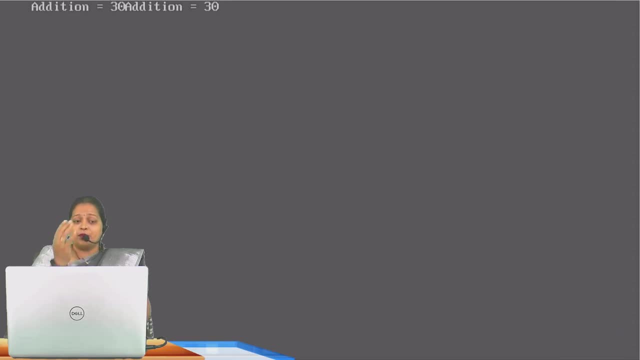 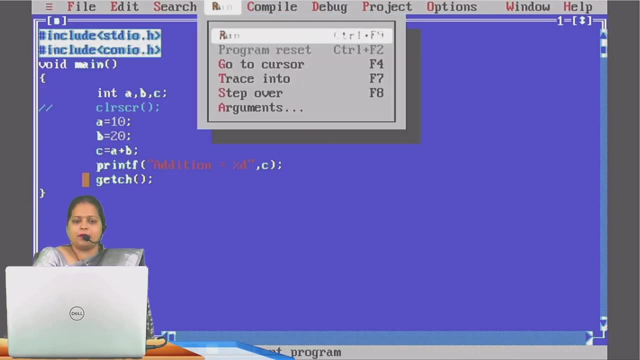 addition is equal to 30. addition is equal to 30. that means you previous mera output addition is equal to 30, or supposed, like clear nick Ria who screen co, as it is a kind of or bar print, execute karuki. we j ip bar de Khaira because a dish.